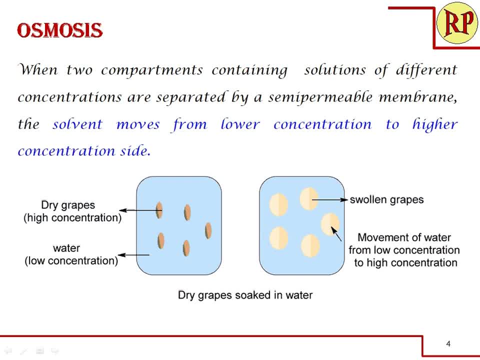 When we soak for few hours, we see that the grapes are swollen. Why does this happen? The water from the compartment moves into the grapes, That is, the skin of the grapes acts as a semi-permeable membrane and the water moves from the lower concentration side to the higher concentration side. this is a natural process. this 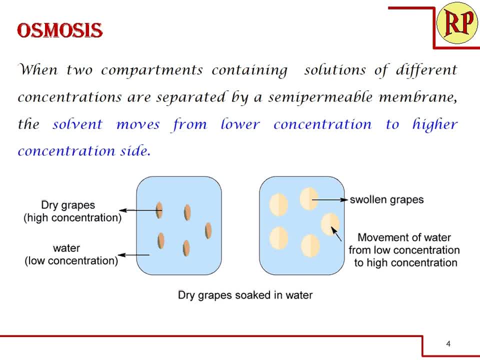 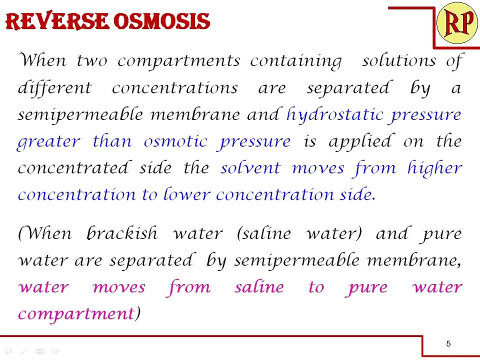 happens with a minimum pressure, which we call it as osmotic pressure. now we are going to reverse that process. this is called as reverse osmosis when two compartments containing solutions of different concentrations and separated by a semi-permeable membrane, and when we apply 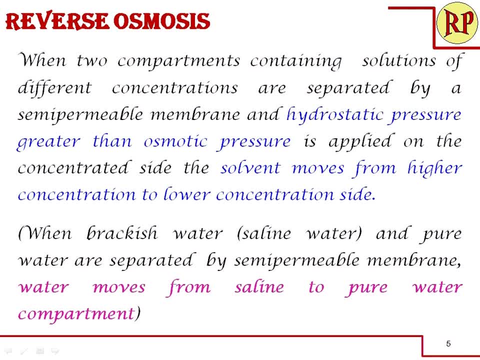 hydrostatic pressure greater than the osmotic pressure on the concentrated side, the solvent moves from higher concentration to the lower concentration side. that is when brackish water or seawater or saline water is separated with a semi-permeable membrane from the pure water. the 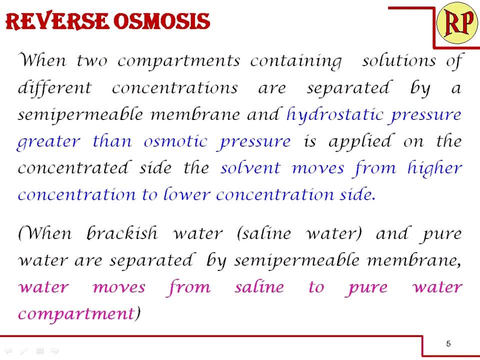 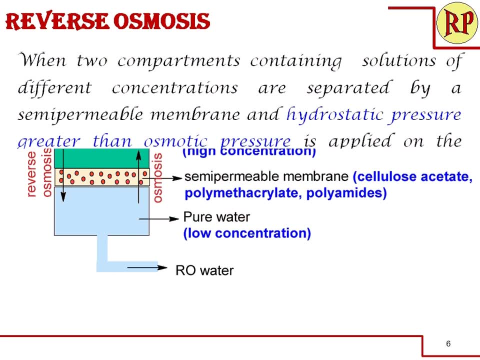 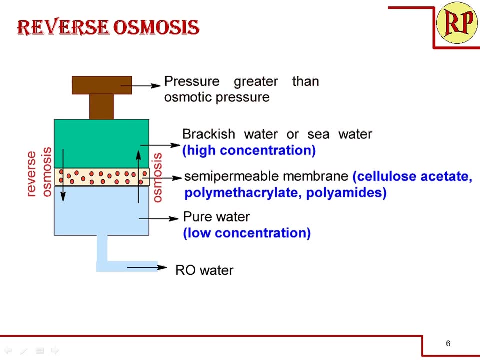 water moves from saline water to the pure water. the water moves from saline water to the pure water, to the pure water compartment, when hydrostatic pressure is applied on this aligned water site. let us understand with a diagram. the compartment with green color is brackish water, which is of 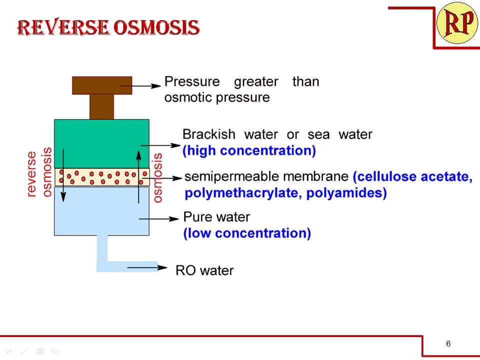 higher concentration and the compartment with the blue color is pure water without away concentration. both the compartments are separated by a semi-permeable membrane which is always found on the saline comes out to the severe moment. the desire has been that this often made of cellulose acetate, polymethacrylate or polyamides. Why do we call it as semi-permeable? 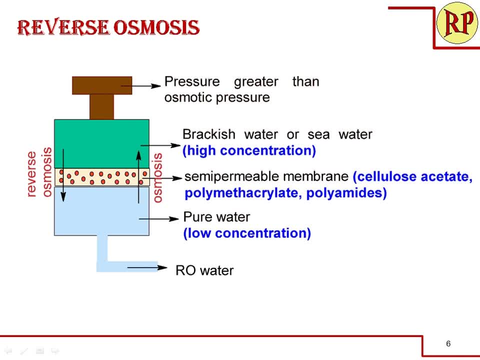 membrane. We call it so because it allows only the solvent, or the water in this case, but does not allow the ions or the minerals or the colloidal matter present in the water When we apply pressure on the brackish water side which is higher than the osmotic pressure.